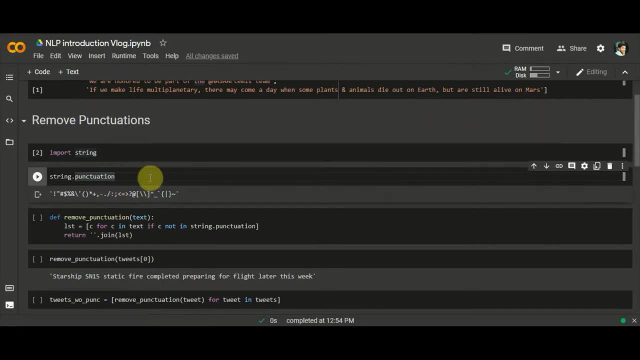 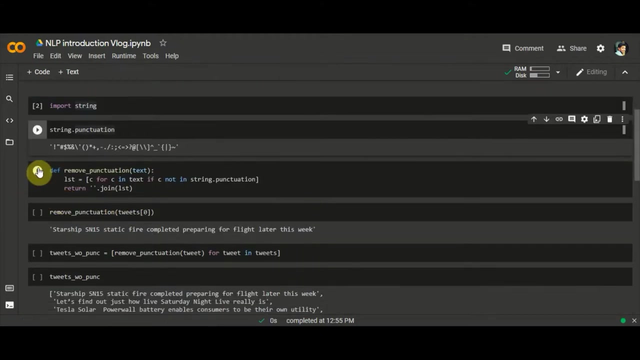 contribute some meaning when a human reads the text, but not for the computer. so it's simply gonna remove that. so we are importing string library and these are string dot punctuation. so I have created a function that takes a text in and returns the text after removing the punctuations from this. so yeah, let's. 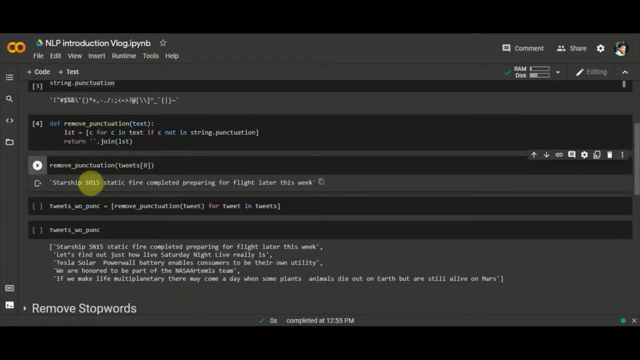 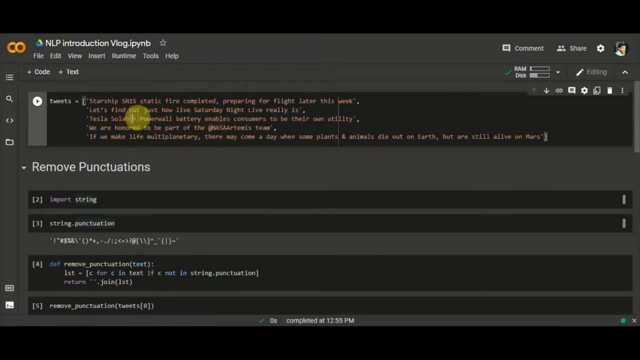 text. our function this is: yeah, so look, you can see there was a comma that got removed here, and let's get all my tweets without punctuations. and this is how it looks like. and at the red from here got removed as well. yeah, this at the right that this plus sign as well got removed. so, yeah, this is the. 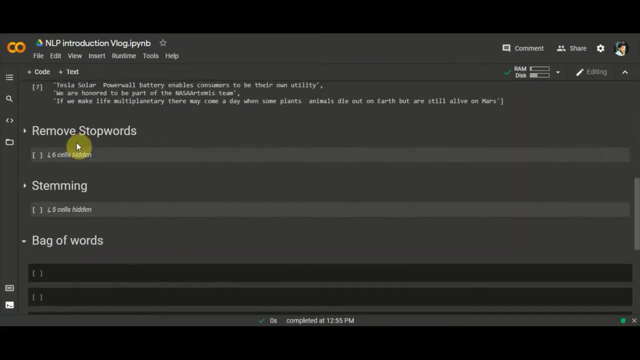 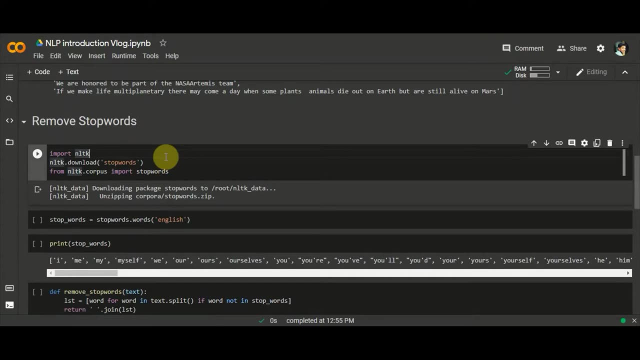 first thing you're going to removing the punctuations. okay. the next step is removing the stop words. stop words are other component of language that plays important role is forming a sentence when it comes to humans understanding of language, but for a computer they are not gonna be very useful. 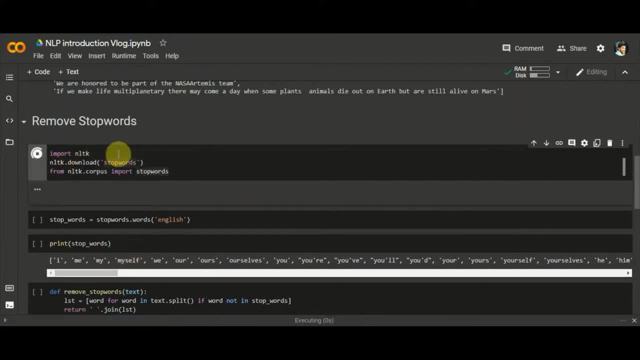 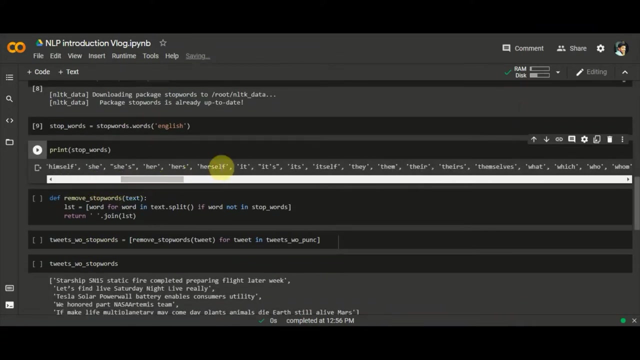 so we are simply gonna remove them. so I'll just import NL DK library- which is gonna be very important for any NLP task, and download in stop words like this and then importing them, creating an object of stop word here. let's print them. yeah, so these are kind of the stop words that's her herself. they're not gonna contribute to people's. 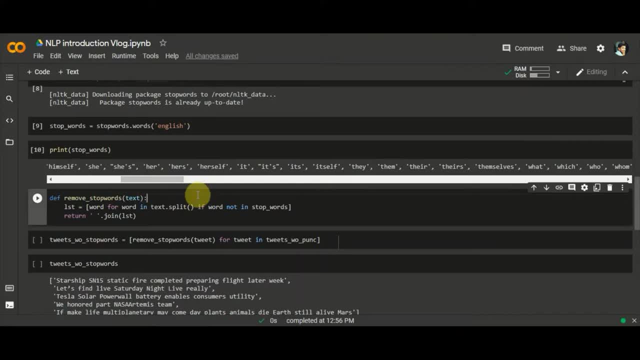 so much meaning to your nlp data set if you're gonna, you know, perform some task like sentiment analysis. when we try to predict how this sentence sound- it is positive or negative- so these kind of words are not going to contribute any information into some words. that's going to contribute the. 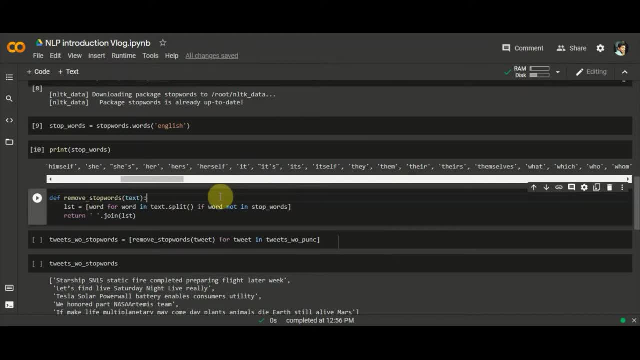 information are going to be like, not, or you know, sad, happy those kind of words are. that's going to contribute in deciding when, whether your data is your text, is positive or negative. so that's why we kind of remove them because they are of no use. so i'll just another function i created. 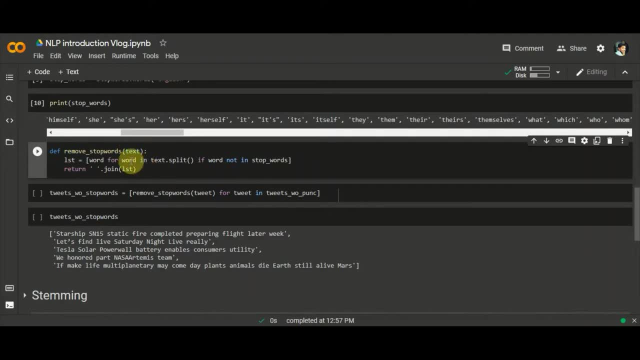 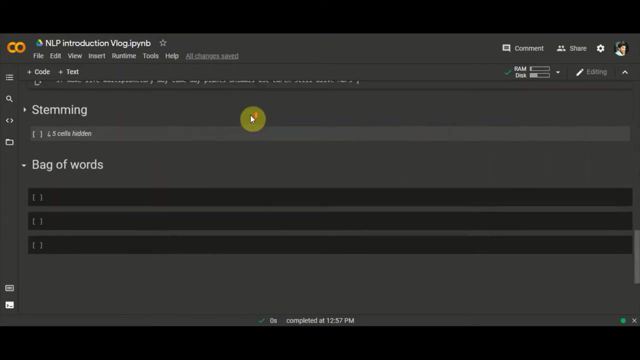 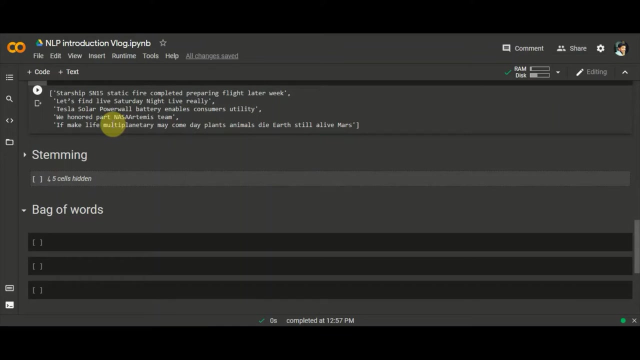 for removing stop words. it takes a text in and removes the stop words and returns the text. so let's get all my tweets remove stop words. and here we are. so this is a data set with: after removing v, honored part. they sound weird kind of. but yeah, it's an important stop a step to remove those stoppers. the next step we have is stemming. 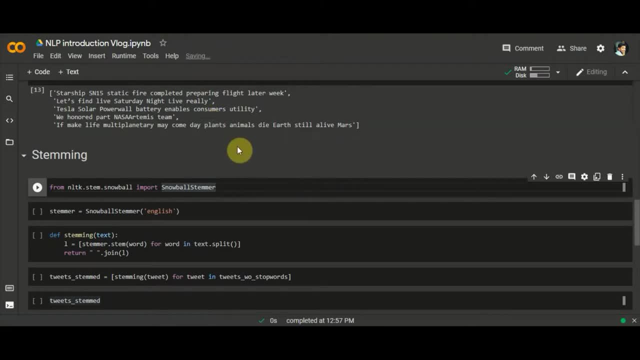 so in stemming we do what: we pick any word and we convert that word in its basic form. so we have multiple form of words in english language. like, suppose: if i have a word complete, it can be found in many forms: completed or complete. you know, second form, third form, any word can be in many forms. but i want my data set. 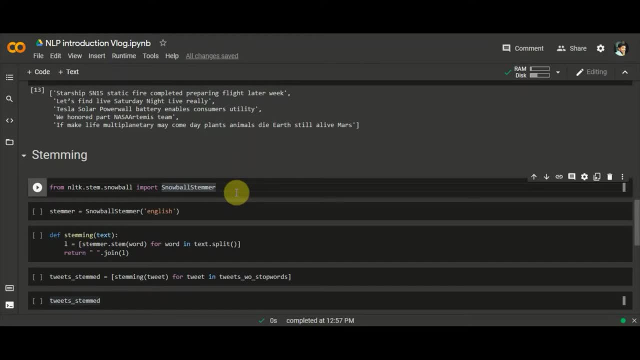 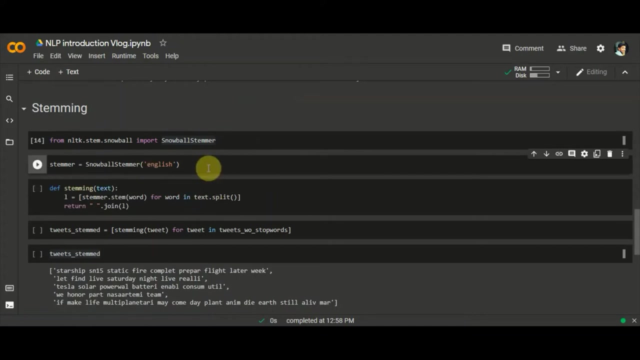 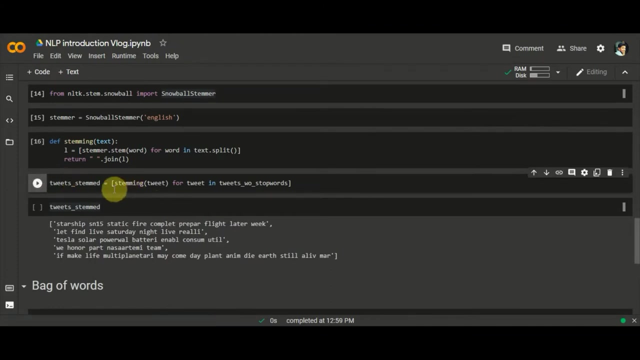 to consider all those forms as a single word, because it conveys the same meaning, all of them. so that's why i'm gonna convert all those words to its basic form. so, again, i'm using nltk stems. we're using nltk stems for the first time and we're using the snowballs timer and creating a object of that, and let's run a function to get all my words stemmed. 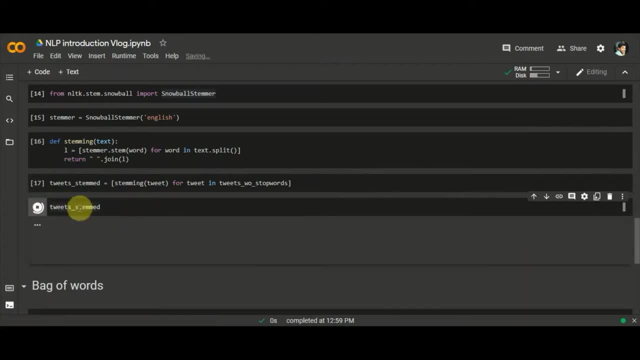 and stemmed tweets. you can see here static fire. complete, this complete word doesn't really mean anything, but yeah, it's the basic form. it could've been complete and now i'm gonna show you how to complete this. completed or complete, it is here. another is: prepare doesn't mean anything, but it's the. 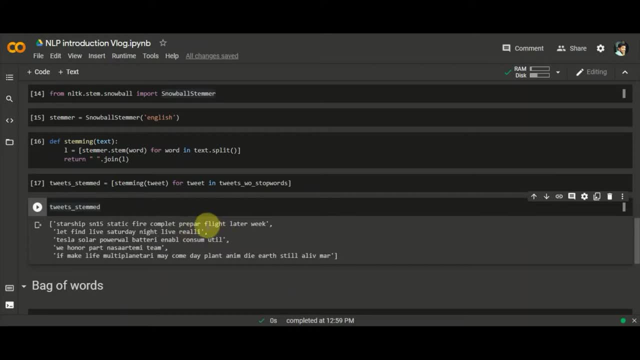 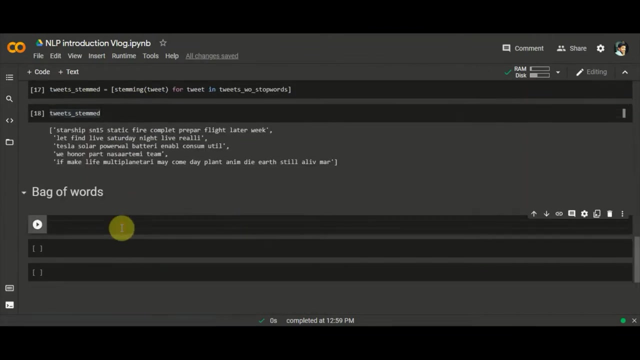 basic form. it could have been prepared or prepare, but they convey the same meaning. so we bring them down to the basic form and we are gonna use them as unique words. okay, so i have my stem tweets and the next step is to count my words. now i have come to in a 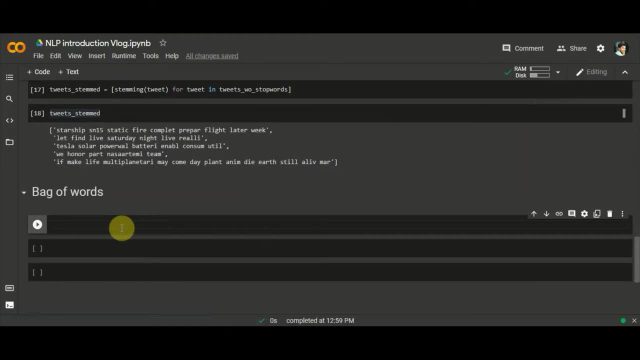 stage, that the final step. we need to convert this text to data, into some numbers, some numerical form. so what i'm gonna do first is i'm gonna find all unique words in my data set. so in my whole data set supports i have these unique words. find, find all unique words. 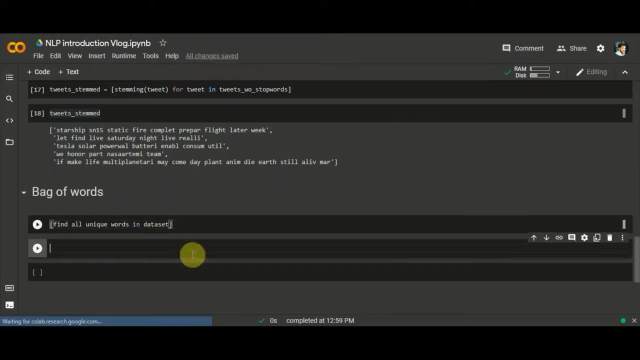 in data set. if i've doze kind of, these are six unicorns, so i need to find all of them first and i need a list of them. then what i'm gonna do for each sentence. i'm gonna write the frequency of my those words, okay, so if find it appeared once in my sentence, so i'm. 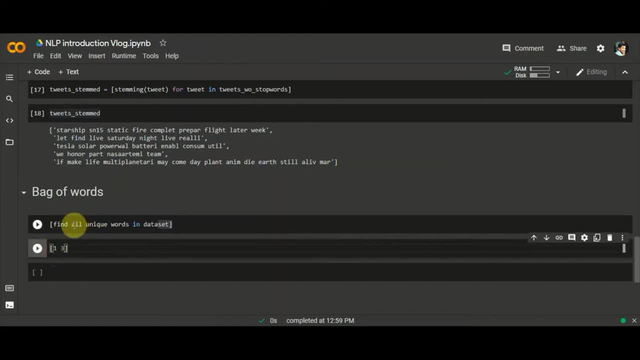 gonna write one for find. if all your has appeared three times, i'm gonna three. and unique didn't appear in my word sentence, so i'm gonna write zero and the other as well, i think. if they're gonna be other two words and in they appear only once in my sentence, i'm gonna write one and data set doesn't appear in my sentence. 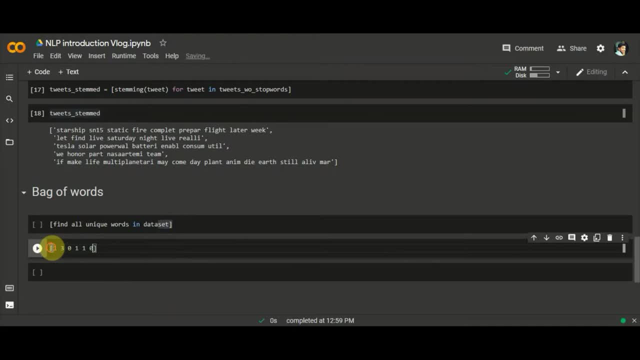 so i'm gonna write zero. so this is how i'm gonna form our data set now. so, yeah, this is how a typical sentence like this would be looking after. final bag of words. you can use count vectorizer from sklearn also for this, but i'm gonna hard code this process, so this would be a coding practice. 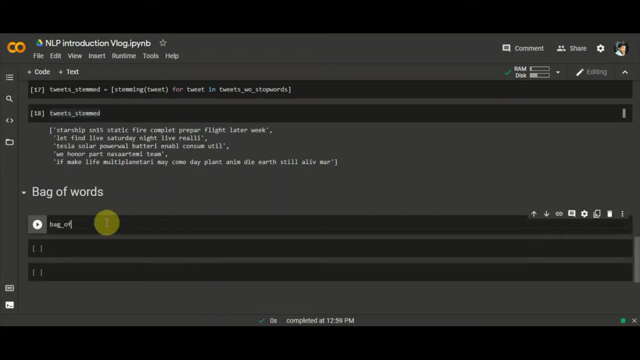 for me as well. so i'm gonna first write bag of words. i'm gonna create an empty list, yes, and in this list i'm gonna put all these words from my data set. so i'll be going through in my data set. tweets stem: yes, because this was the last step we got. so after tweets stemmed. 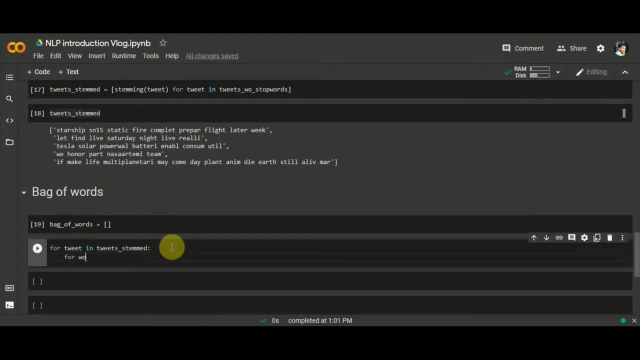 in each tweet. i'm gonna iterate through a word and in each tweet, so let's split by spaces and it's gonna return a list of word and for each word, what i'm gonna do: i'm gonna append it in the bag of words list, simply so, yeah, let's run it now. check my bag of words. 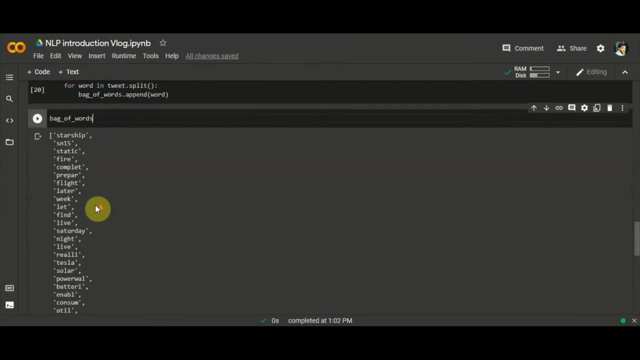 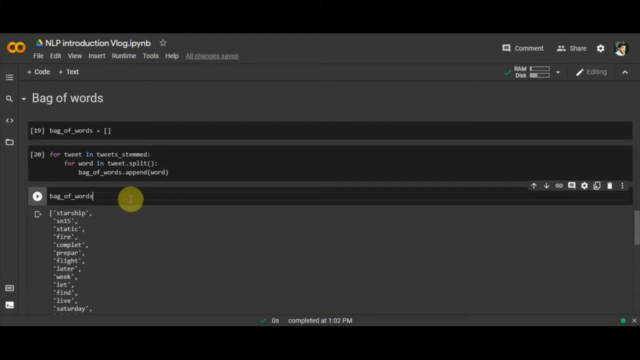 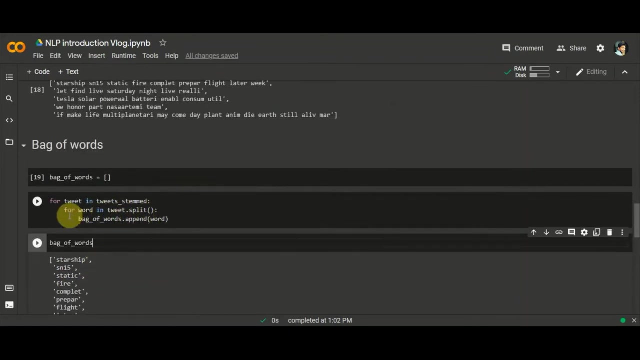 let's see. cool, i have my words in this list, but we're not done yet. not because there can be multiple words as well. you know, one word could appear multiple times because we haven't taken care of the duplicity. there can be duplicate words, you know, and we wanna we. 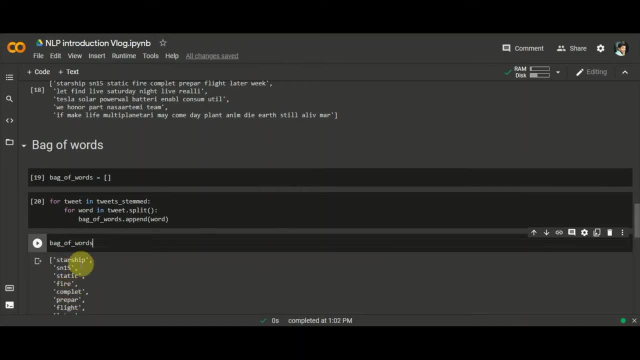 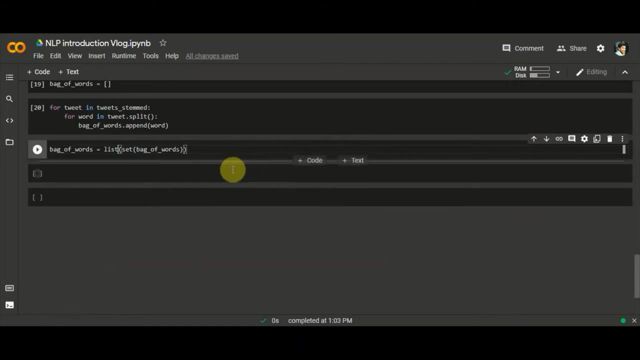 want one word appear only one time in our list. so I'm just gonna make a set of this bag of words, which is gonna give me unique values, and make a list out of it again. so yeah, now my bag of words is completed, so the next thing I'm gonna do, 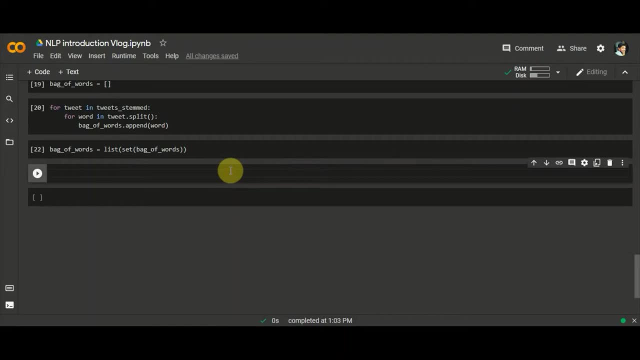 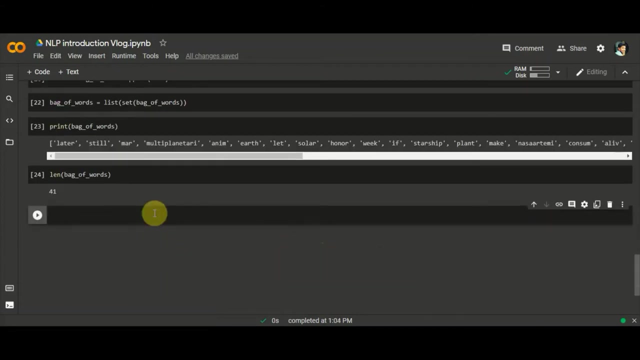 is. now I have to count. let's one more time print my bag of words. so now for each of the. okay, I have the list now. okay, all words are unique. let's see length of 41, cool. so. and let's have data as well. so its stem. so, for each of this sentences, these tweets. so what I need to. 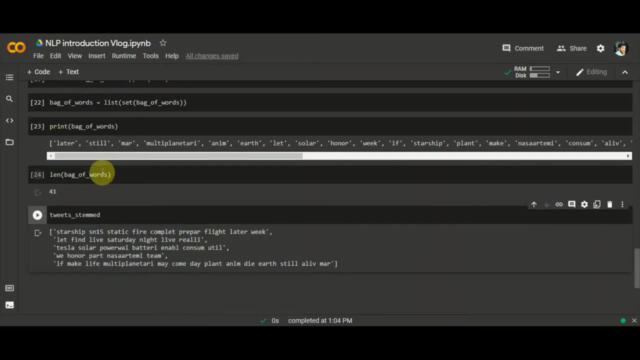 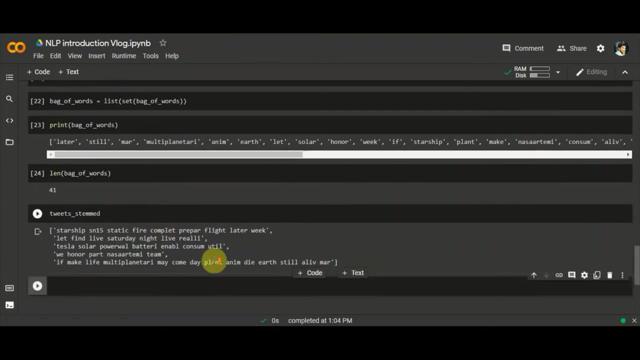 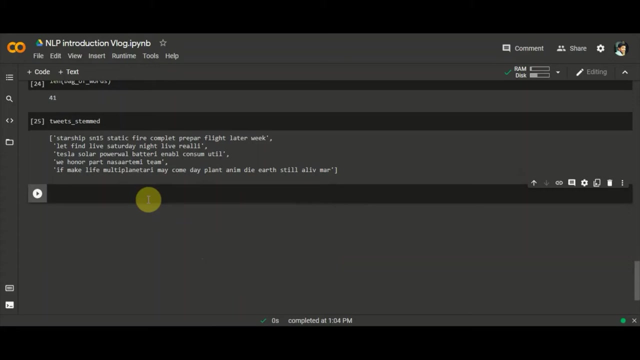 do now. I need to count those words and make a data set. as i shown a minute ago, i need to count and by the frequency of those words i'm gonna make a data set. so yeah, let's do it first. so i need to. first i'm gonna use dictionaries. you can also do something like this. 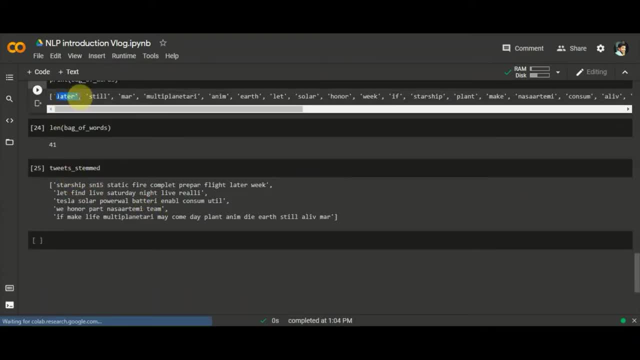 you can go through, iterate through all these words and for each word you can go through all a sentence and count its frequency, but in that time complexity would be there. i'm gonna use a more efficient way by the use of dictionary. so yeah, let's look at this. so first i'm again. 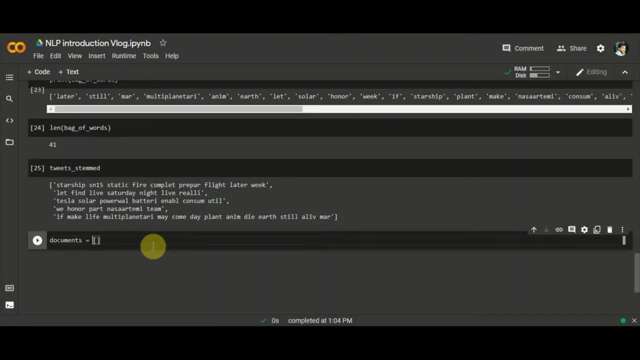 making the list, that which is documents. so this is gonna contain my all of the converted data in numerical form. so in this document i'm gonna, this document is gonna contain dictionaries. a dictionary is like, would be like it would have word as unique, unique word as a key and its frequency is 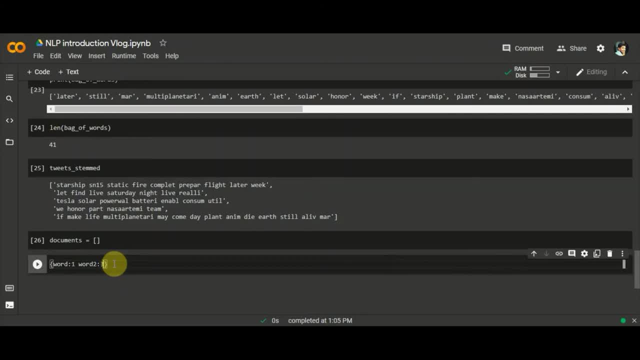 and something like this. so for each of my tweet, i'm gonna create a dictionary like this and that. that dictionary i'm gonna store in this document. so let's get started. for again. tweet in it's 10. yeah, i'm gonna create an empty dictionary. not an empty dictionary. i'm gonna create a dictionary with. 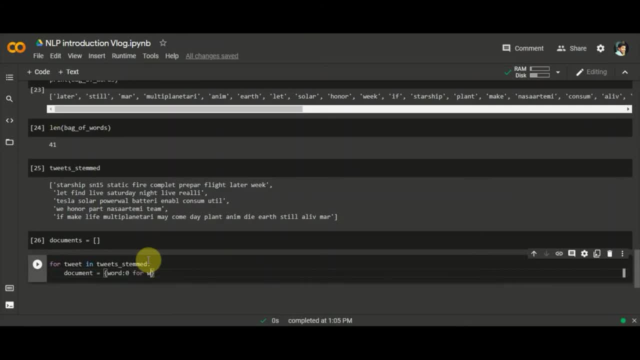 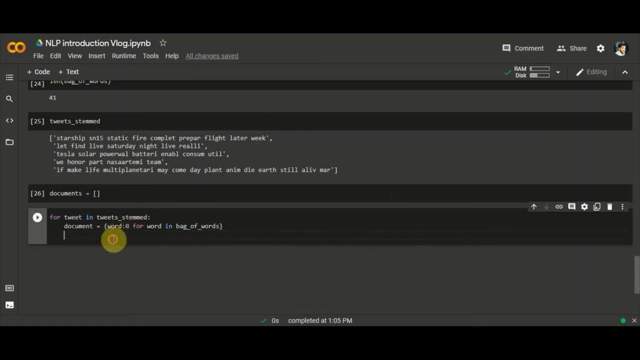 a word and count. i'm keeping zero for word in my bag of words. so all of the this will do what. this will create a dictionary with all of my unique word as keys and their count as zero. and next i'm gonna do what. next i'm gonna. 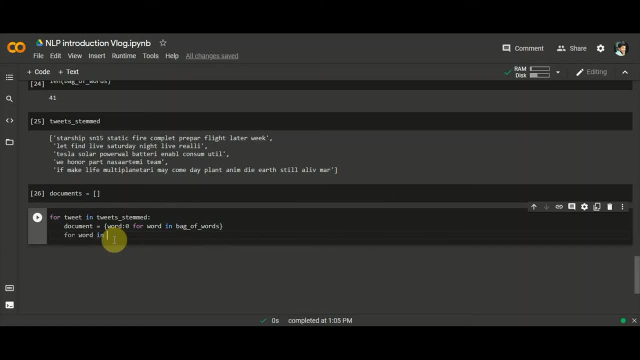 iterate through each word in sorry, in my tweet, each word, and i'm simply gonna increase the count of that word in my document dictionary by one. so in this way i'm gonna get count of all and, and finally, i'm gonna store my document in my list of documents. 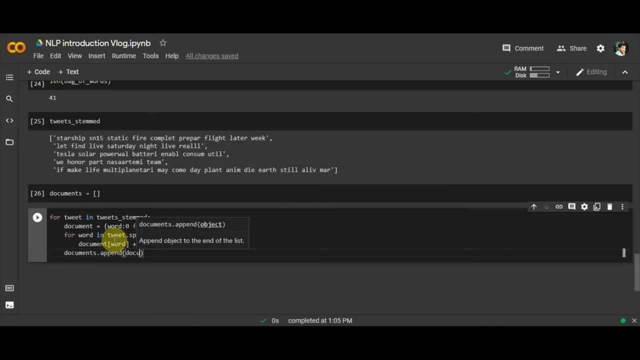 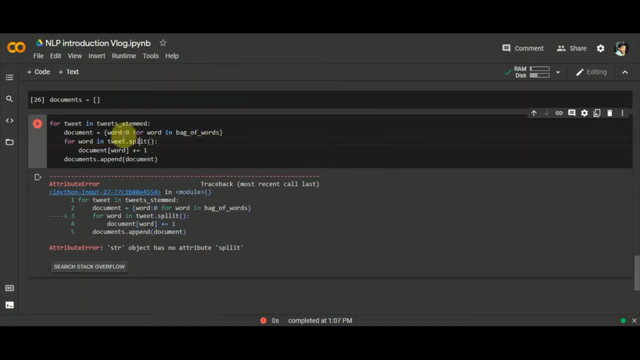 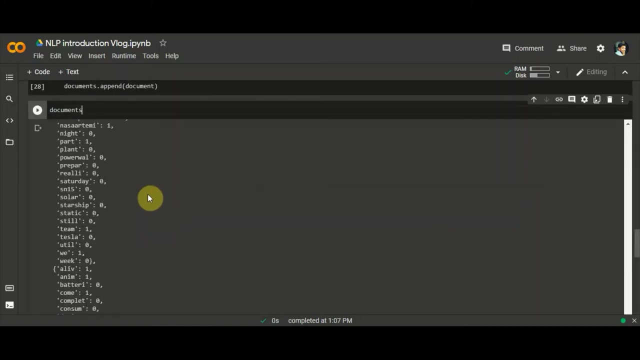 by append method. so document, let's run it. hope we don't get any error, but we've got okay, but this should be split with one l: yeah, now cool. so yeah, let's see how our documents look like. cool. so we have five dictionaries. see alive zero. some words are one because they appeared once in. 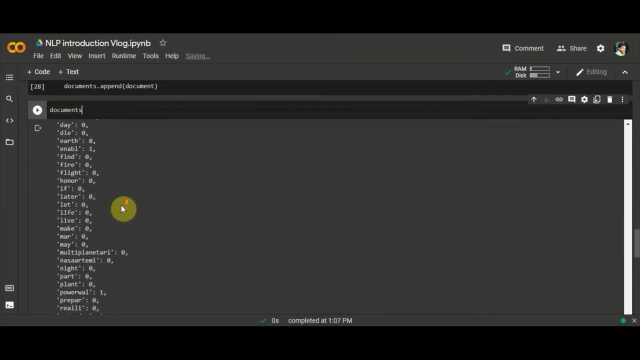 our sentence and yeah, cool, so this is how it looks like. so, yeah, we are almost done with the data set. now let's convert it into a data frame to view it in a tableau form. sorry for that data frame equal to pd dot. so i'm gonna take a list of and for list of. 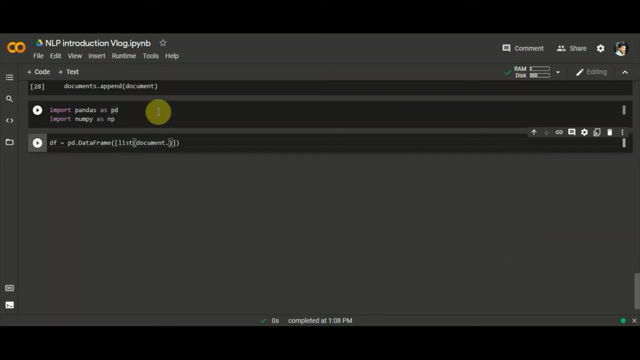 document dot values, document documents. so i'm taking from documents, i'm taking each dictionary and its values. i'm i'll be taking as rows, and next i need columns. so my columns would be list of documents, zero- any element i can take- and keys, because keys are my unique words. okay, so this. 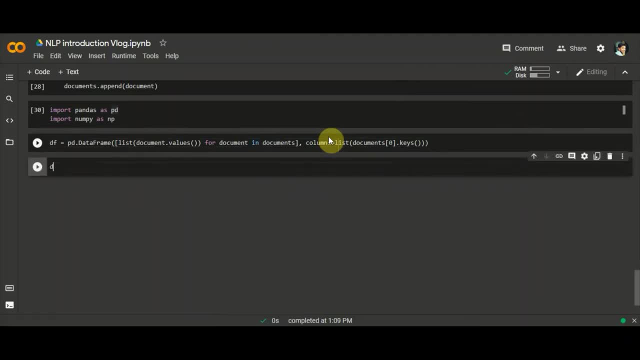 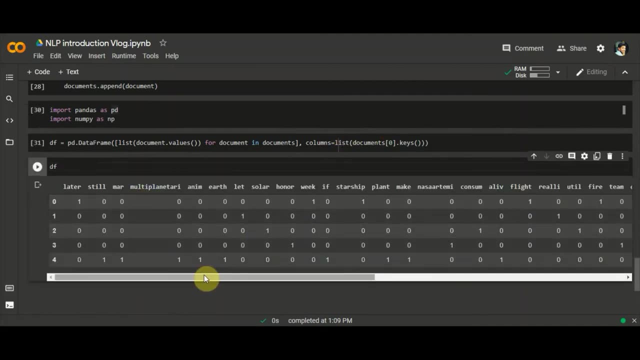 should work. let's run it. okay, cool. let's see my data frame. now. this looks good. we have our unique words as columns and- and, yeah, their frequency in the sentence or tweet as the rows, as values. so you can see most of them are zeros, but you can see live in the second tweet, live comes two times i think. let's check it.